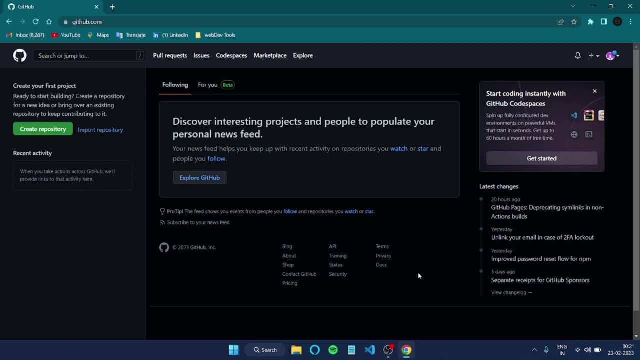 hey guys, welcome back today. in this video, we will know how to deploy our static website on github. okay, so, if you know, this, github is actually a platform where you can upload your projects and you can even collaborate with other developers. okay, so this is actually a must-know technology. 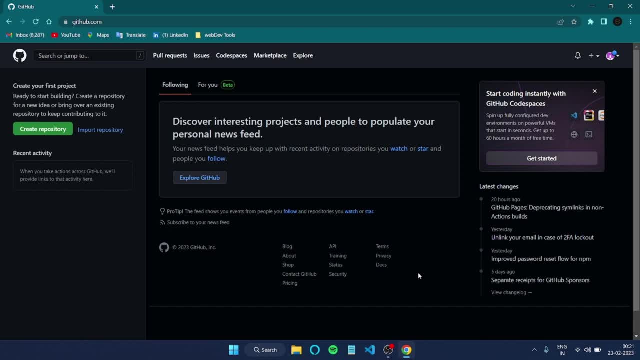 in 2023 and even in the future also. uh, there are other platforms also, but this is the most widely used one. okay, so here in github, we can deploy only static websites. okay, so we can't just, uh, deploy our dynamic- also dynamic in the sense which has apis and all- if you are performing any kind of. 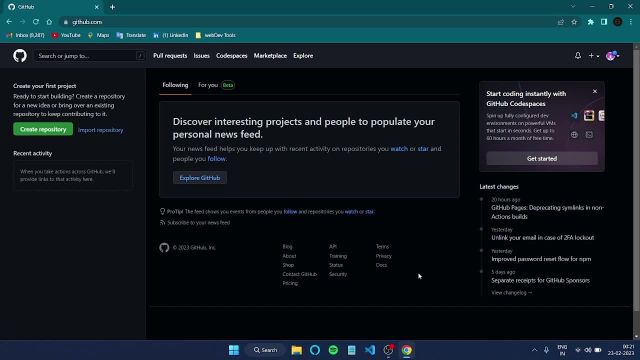 get post operations and all uh apis and all you can't just upload here, uh, deploy, okay, so this one is for a single page applications, okay, uh, anyways, we'll just get into the video straight forward. so first of all, you need to create a account in github by by now, i believe you. 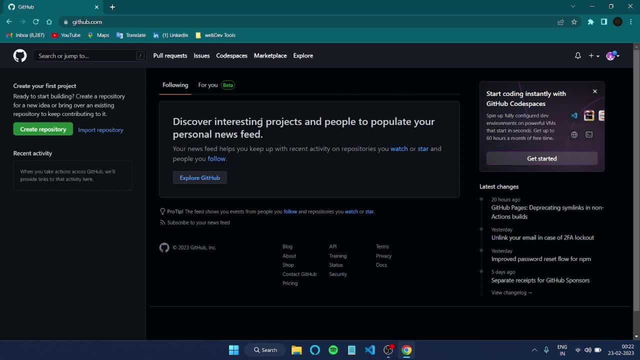 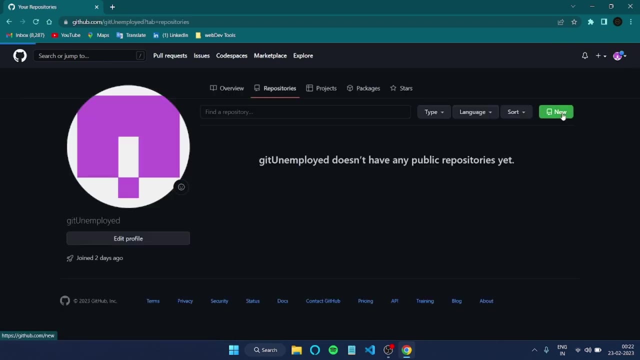 might have already created the account, okay. so first of all we need to create a repository, okay, uh, to create that repository, okay, either you can click directly in create repository or there is option: uh, profile and your repository. here you can create a new. okay, then you have to give any name here. for example, i'll be giving here test, okay. 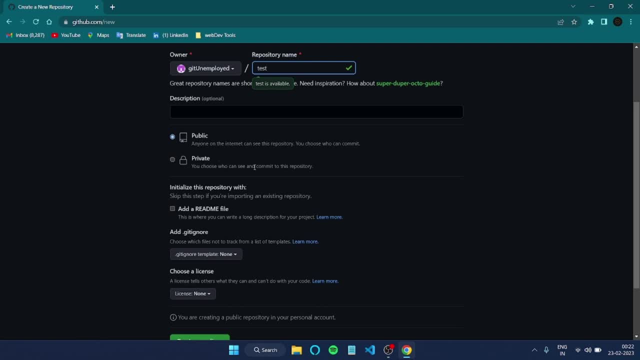 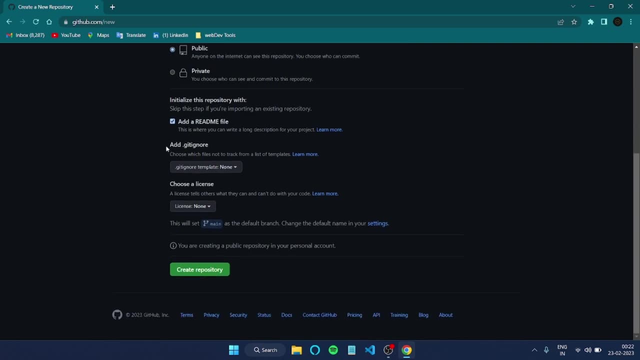 uh, this can be any name. i choose whether this should be a private or a public one, okay, so then, uh, it's better to add a readme file, okay? so, uh, what happens in readme file? you can explain your project, what and all uh steps you have taken. you can just, or you can just, give an overview of that. 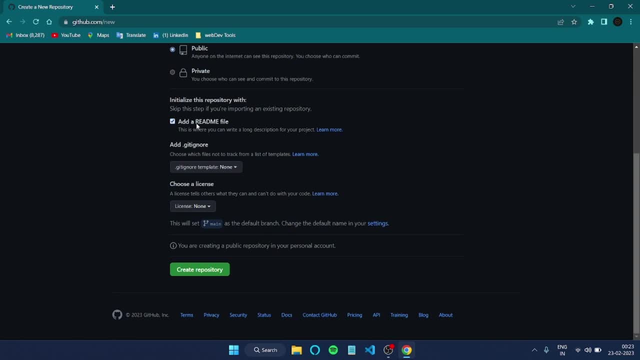 project. okay, so it's actually good. um, it's always a better idea to give a readme file also, so the whoever the viewers is coming to see your projects now, he will understand by reading the readme file only. okay, so after that we have to click on this: create repository. 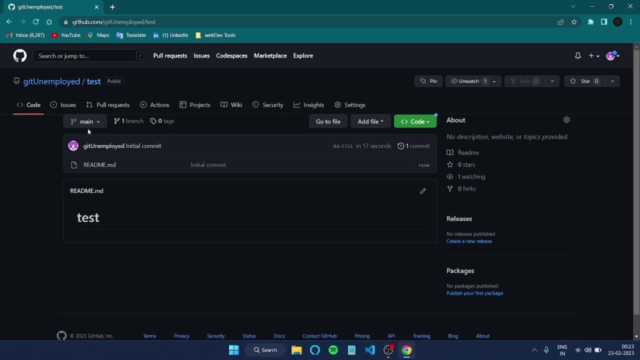 okay, so after that, now the repository has been created, you can see: uh, this is my repository name: test. okay, so in order to uh use this one, i have to click on code and in https, i have to copy this link. okay, so after copying that one, you need to just get into your vs code. 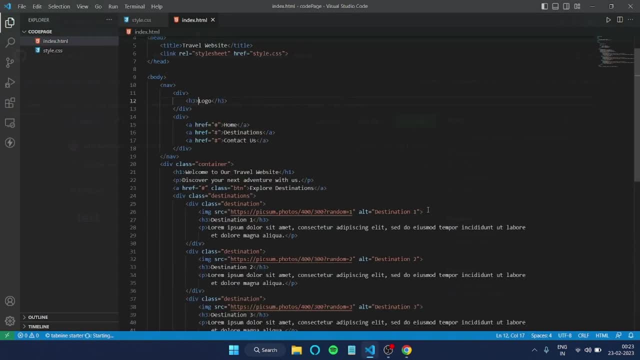 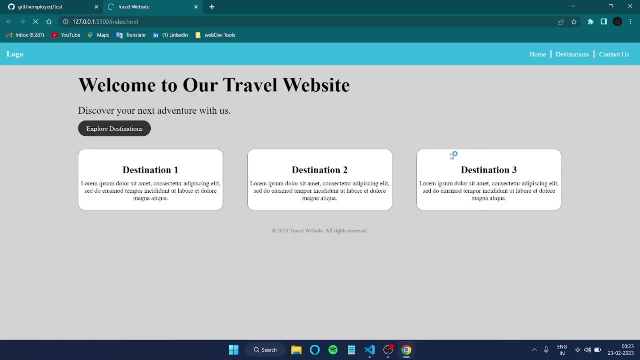 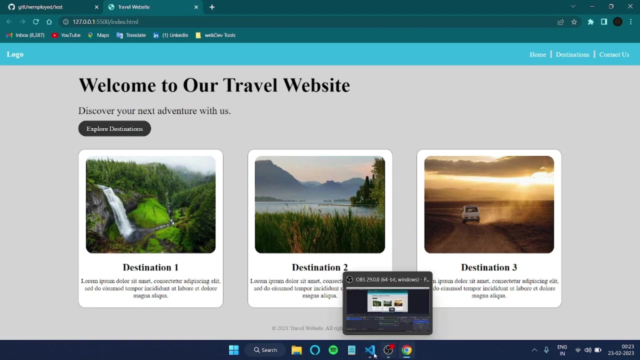 okay. so i have created some uh basic uh, which is nothing but a simple. i will show you: uh, this is a simple uh single page website. uh, no much, uh, just i, i did just for this uh video only, okay, uh, so then after that you have to open your terminal, i'm just okay. then, uh, here you have to. 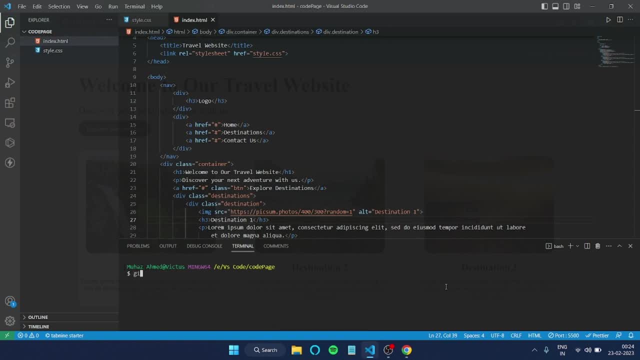 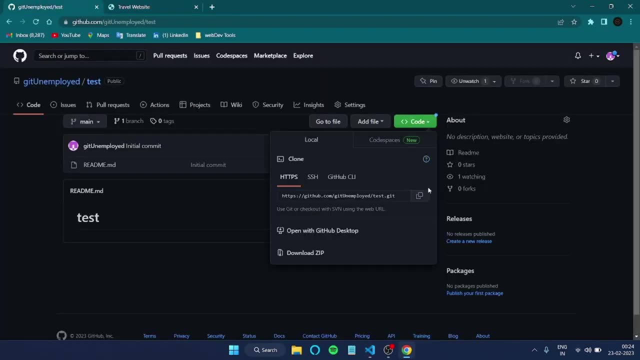 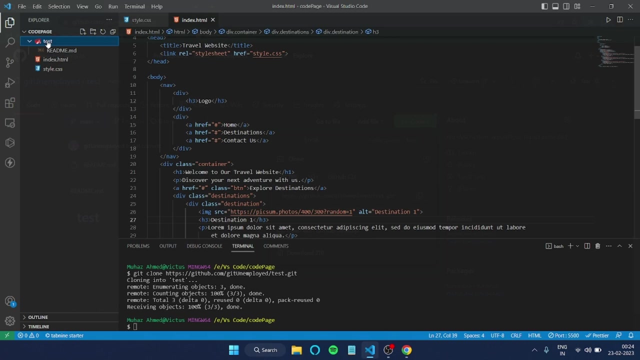 type a command: okay, git clone, and you have to paste that. whatever the link you copied, know here in which the the copied link, you have to paste that here and click enter. okay, now you can see. uh, there is a folder created inside here. okay, now we have to move this for. 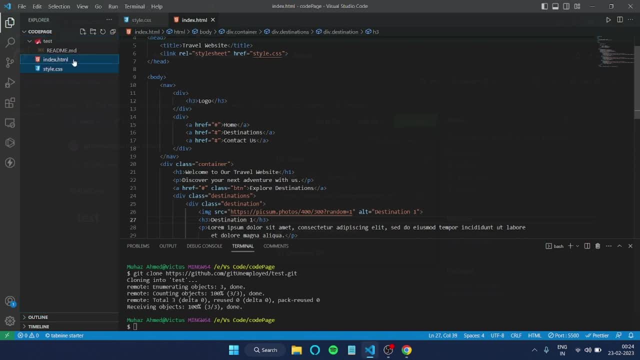 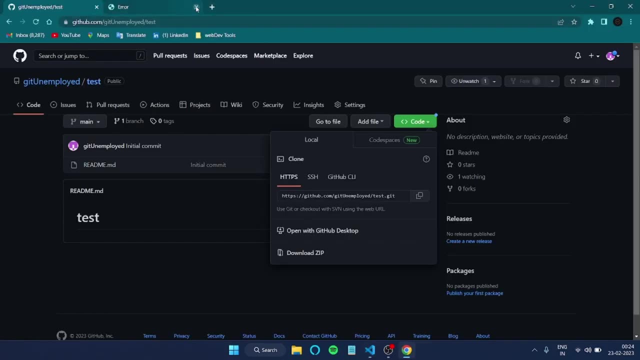 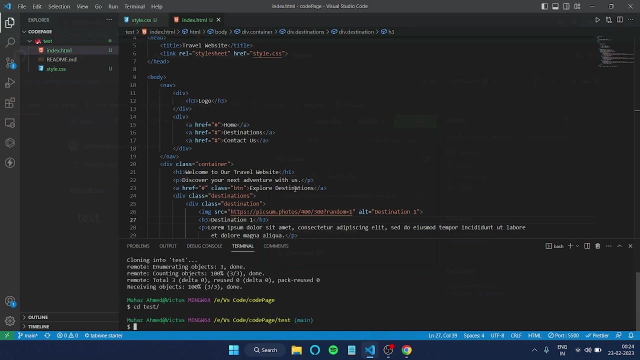 files into these two files into test, okay. so yeah, i'll just stop the server now. i'll get into this cd test and let me close this one also. okay now, if i run the server right. so if i go for a live now, you can see the same thing is going on again here. 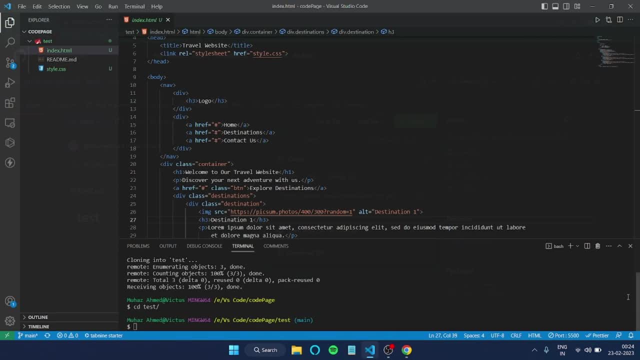 okay, so after that, now we have already inside this repo. okay, now we are inside this repo. now we have to push that. whatever the code we have written here, right, we have to push that in our uh github. we have to make it public so to. in order to do that, we have to give few commands like git add. 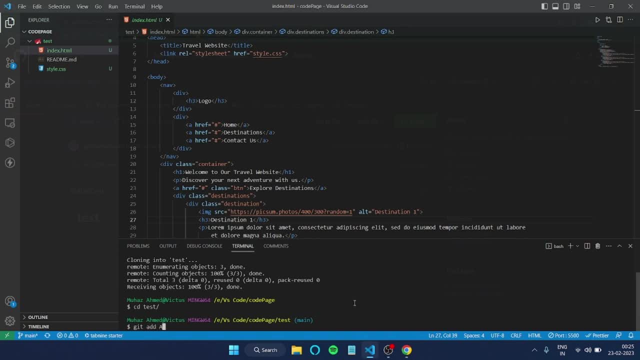 uh, you can give either dot or capital a, both are same. uh, by doing this, all the rep, both the files will be added, both. whatever the files are there uh need. uh, all the counts of the files will be added. okay, so after that the next command will be: git, sorry, git, commit hyphen m. then you have to give a message here, or this is: 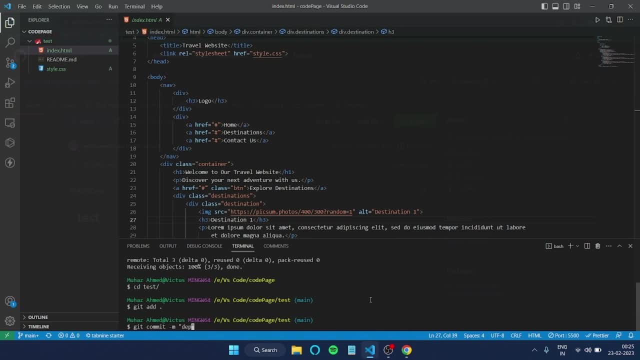 a. you can give any kind of message, i'll give deploy. okay, so now you've got the messages also. now that we have given the message also now the next command is to push the code. to push the code. uh, as a, as i pronounce right now, the same thing, git. 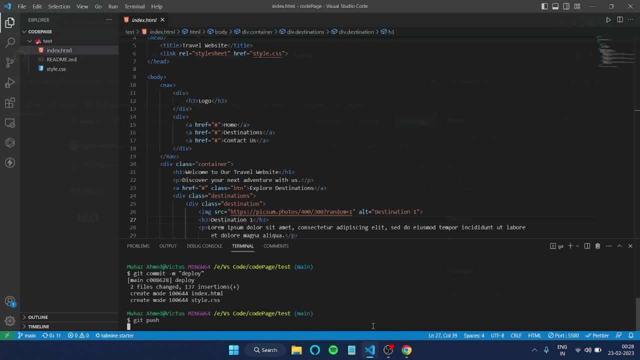 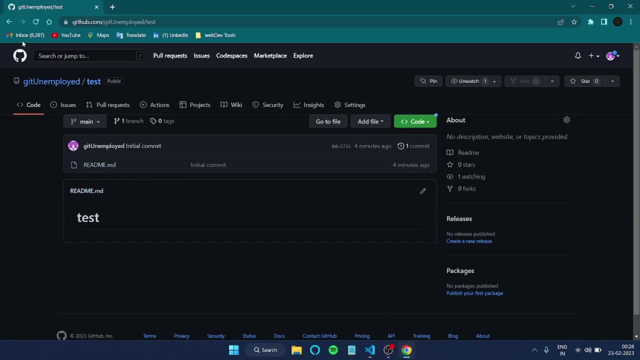 push. okay, by doing this one, you will be able to push the code into our git repo. okay, now it is got. uh, push. you can see now there is nothing here. if i refresh this page, the two files got added here- my html and my style- and it is correct. now that's what we have here. okay, now let's go into our code. 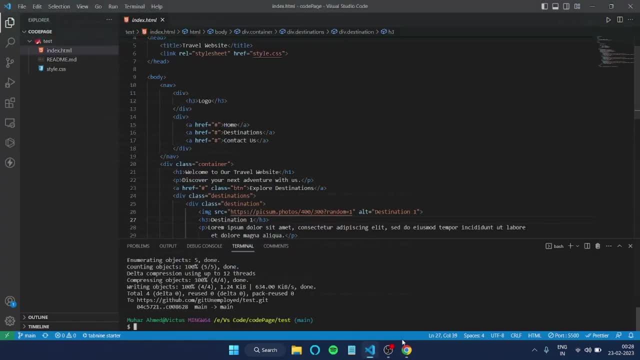 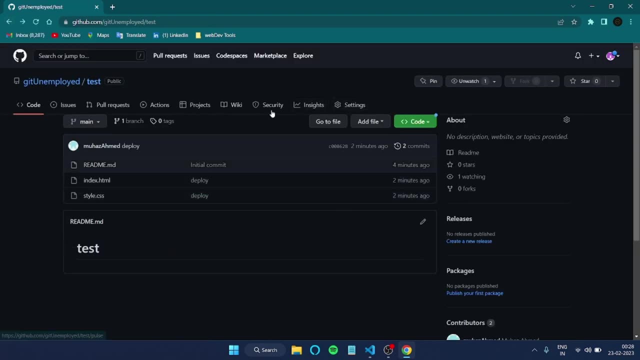 stylecss. okay, so there were only two pages that both also got added here. okay, so after that, now we have to publish this. sorry, we have to deploy this right. so in order to deploy this one, which is our main part, we have to just go in here. settings- okay, you can see your settings okay. 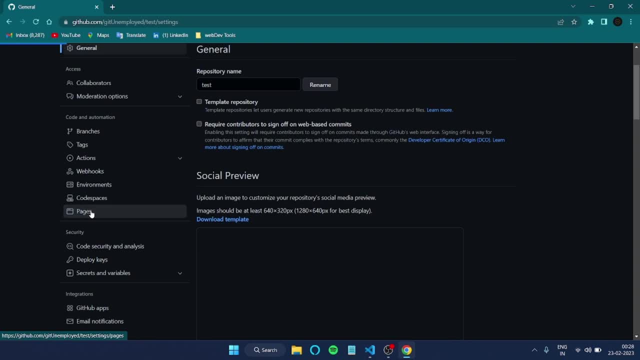 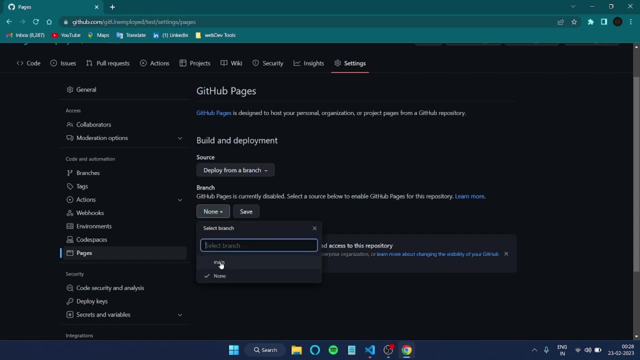 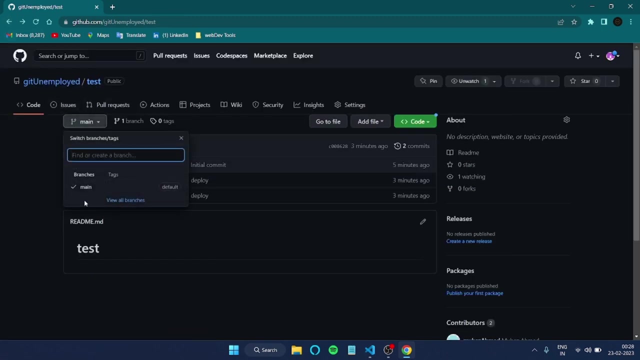 so after that, just scroll down a bit and you can see your pages. you just click, click over that and here we have to give a branch. right now we are in a main branch. okay, i'll show you for example. okay, so this is called main branch. if you have created any other branch, 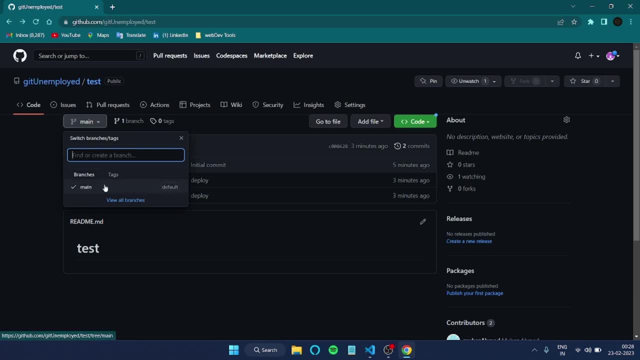 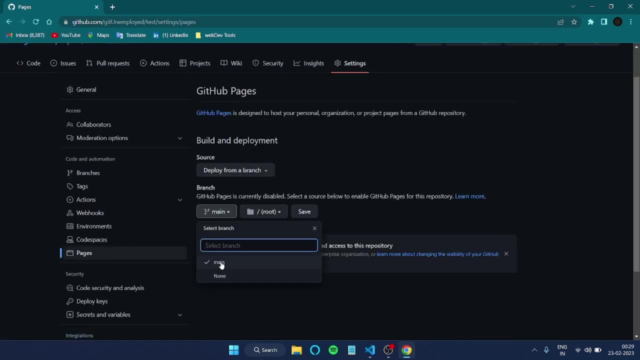 like, if you are giving any there, this is a default one. okay, so if there is any other branches, you have to specify that one. okay, so now we are in a main branch, right, so i have to give main here. then if you are inside any other document, like another folder, 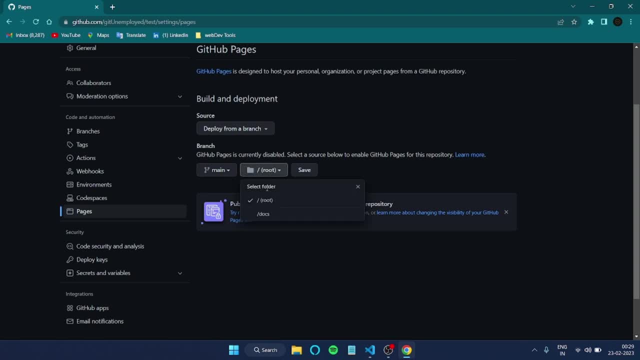 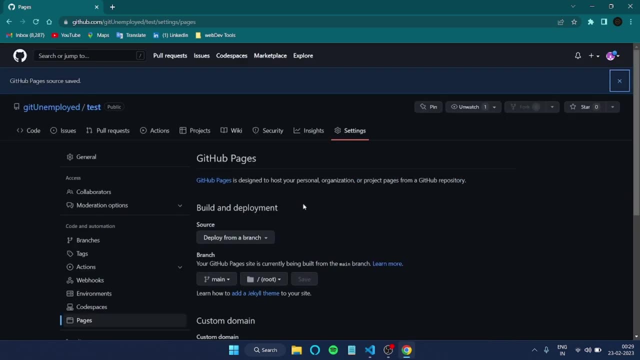 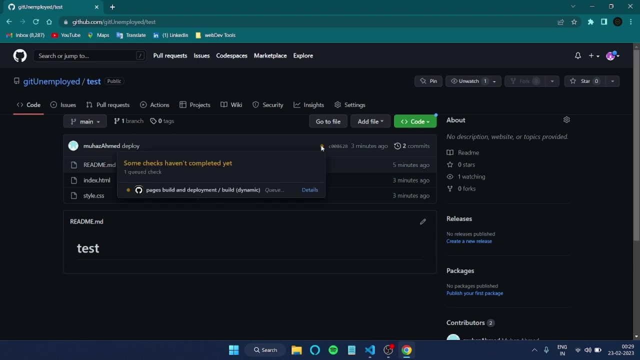 you have to specify that also, since now we are in a root folder, i'm giving root only then we have to click save here. by clicking save, our site will start to deploy. okay, to check that, you just come here into code and you can see a small dot here, right, you click over that and details. 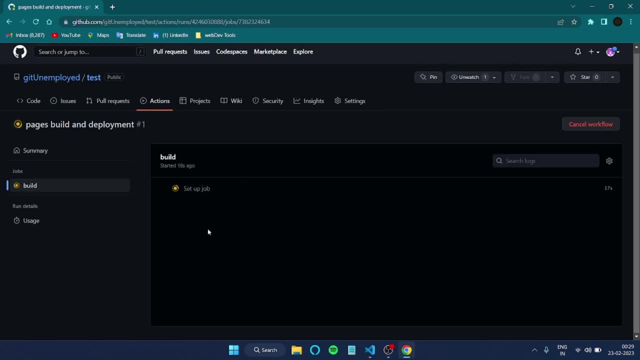 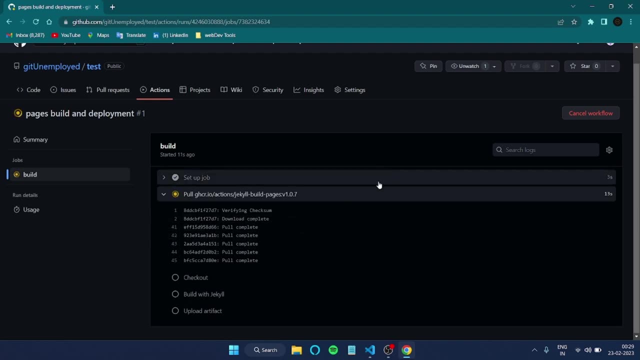 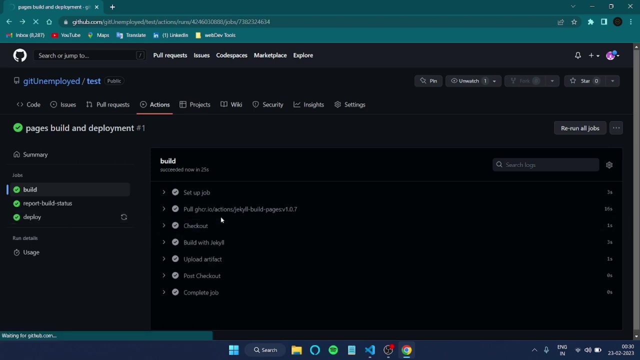 now you can see whatever the logs are going on, right? uh, those, you can just uh cache those datas here. only if there is any error it will show here. only, okay, so we'll just wait until this get completed. okay, now, our site got deployed right now. okay, you can just open this one. you can just check here. 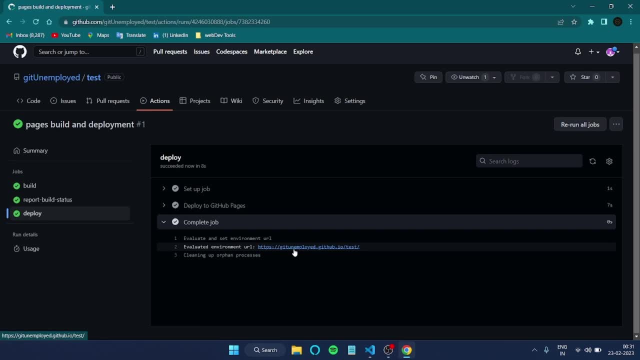 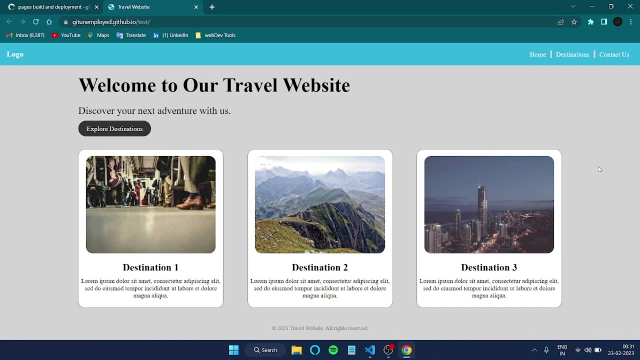 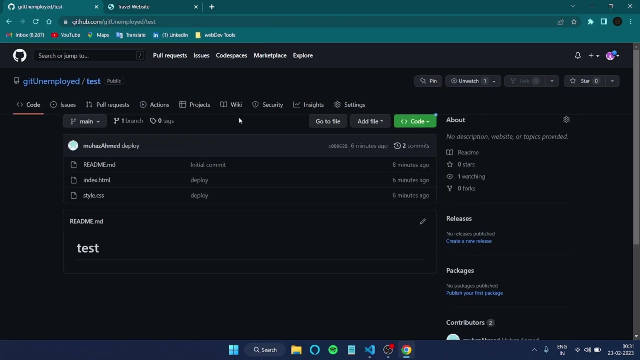 in a evaluated environment url. okay, you will be getting a short link here. you can just click over that and you can see the server is now. whatever the project was there, it was public deployed and don't forget, this works only for the static websites. okay, if you're having any kind of apis and all, it won't work.